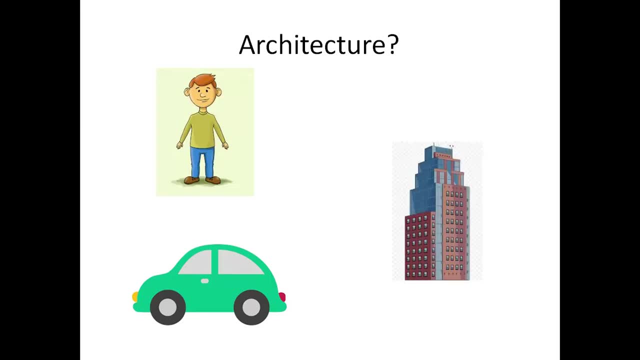 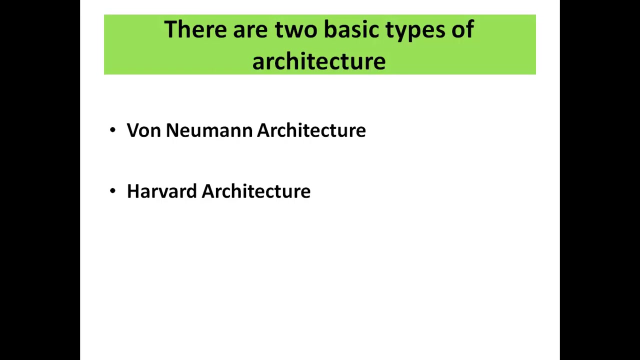 architecture. car has its own, and even building and offices has its own architectures. architecture defines how function works. the same way, the computer has its own architecture on which computer runs, architecture also known as computer model. so there are two basic types of architectures, that is, von Neumann architecture and Harvard architecture. so let's first of all we 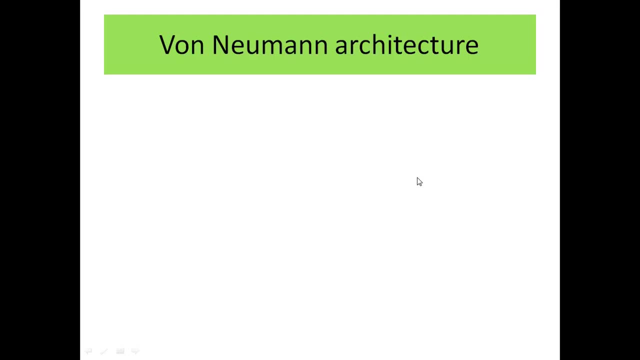 discuss von Neumann architecture. von Neumann architecture was designed and developed by great mathematician and scientist John von Neumann in the year 1945. most of the complete rough today's word are run on Warren human architecture, whether mainframe or person, computers, so von. 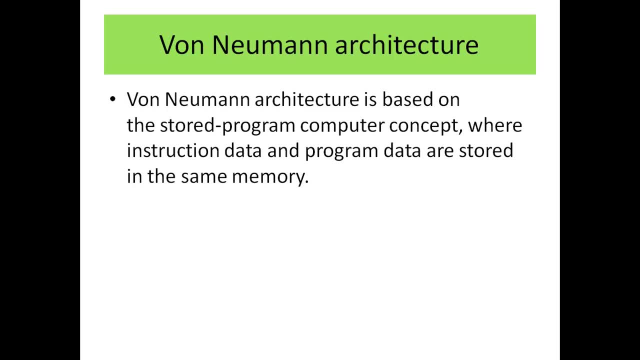 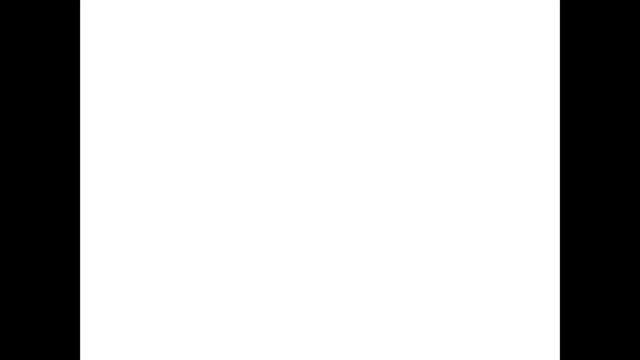 human architecture is based on the stored program. computer concept, wear and program data are stored in the same memory. it is also known as stored memory architecture. so what actually meant by stored memory means that we generally keep two items in main memory, that is, data and associated programs, or you can say that set of instructions. the cpu can be either: 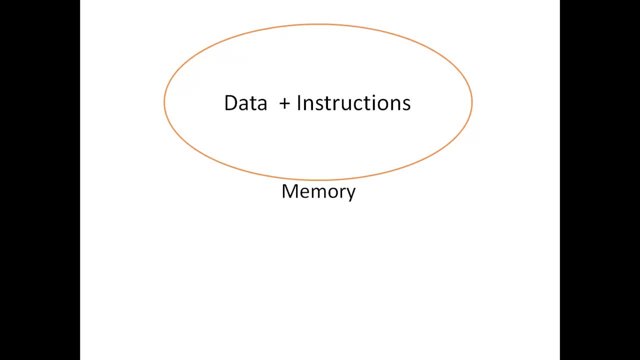 reading an instruction or reading writing data from to the memory, because instructions and data use the same bus system. data means which we have generally write in our normal high level languages like int: a is equal to 10, b is equal to 20 and c is equal to a plus b. it means all those variables. 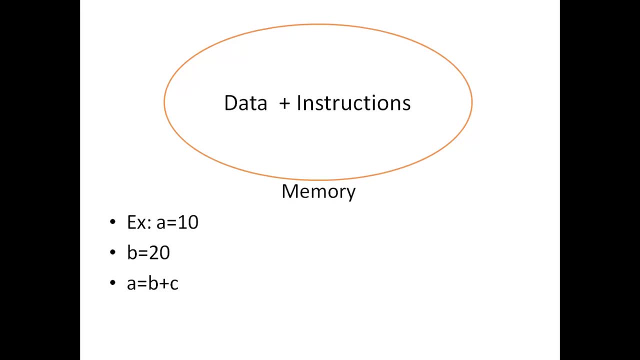 which we are defining are basically used to store data, and these are all available in main memory. and secondly, we store programs, or you can see that set of instructions which explain us that how to do the particular task. we have different types of instructions, like mov for moving instructions. 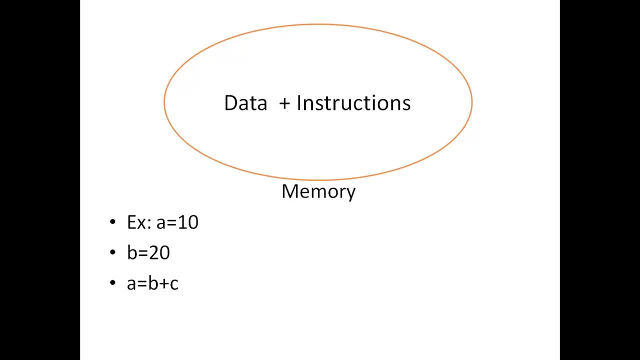 awd, add for adding, sub for subtracting and other branch branch statements also. so all these commands and associated data we generally keep in our main memory, although we can place instructions and data at different locations or addresses in the same main memory. but if we compare it with the harvard architecture in which in this we keep instructions, 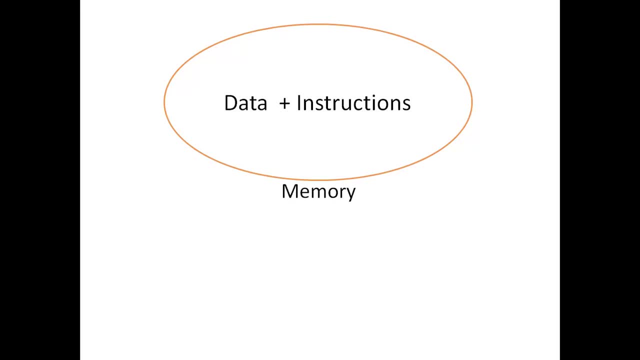 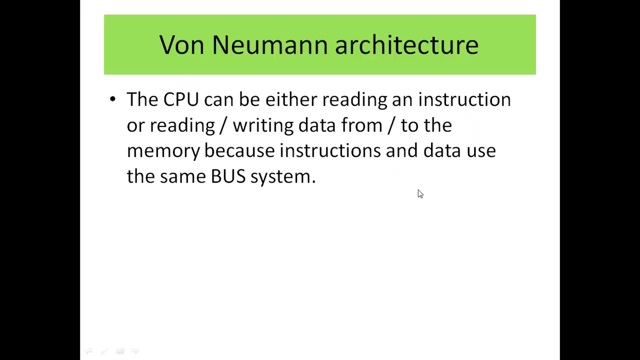 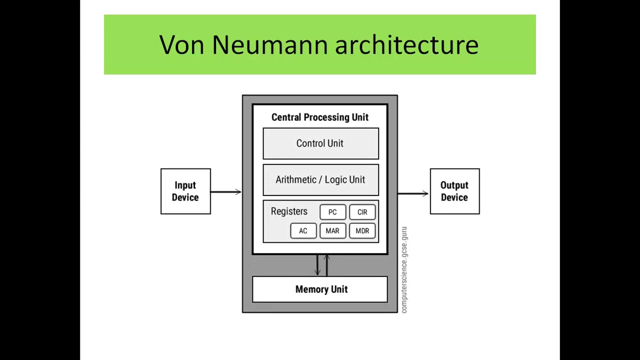 set in different memory and data is in different memory. but in von neumann case we are keeping both data and instruction in the same memory. so this is our von neumann architecture. it is a general architecture which we have already studied in fundamental of computers. it is consist of different units, or you can say that different. 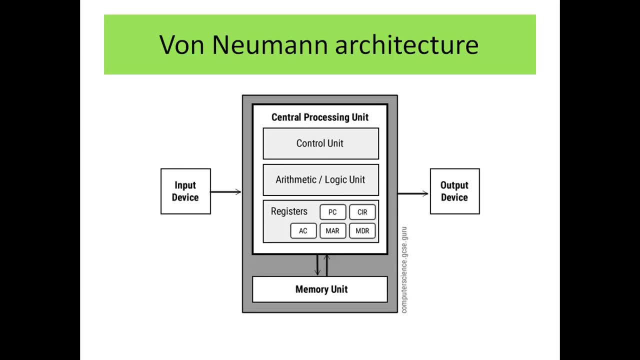 components like there is input unit, processor unit and output unit. processor unit is continuously, continuously in touch with memory unit, from where it takes data and associated instructions. so this is our von neumann architecture. cpu is consist of three parts: that is alu cu, that is control unit and registers von neumann components. 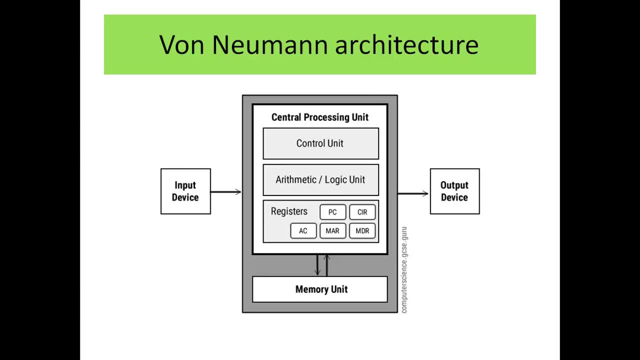 in this architecture also tells us what are the basic components of von neumann architecture that help in processing data, that is, converting data from input to output. that is first, main memory in which we keep our data and instruction. next we have cpu means central processing unit. this is the place where main processing take space. 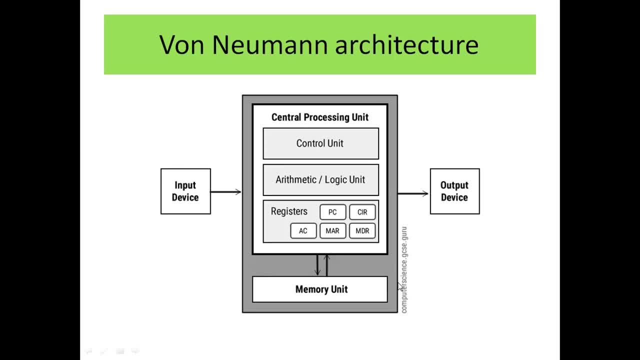 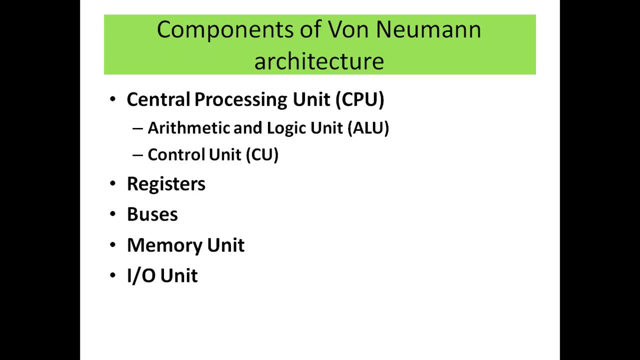 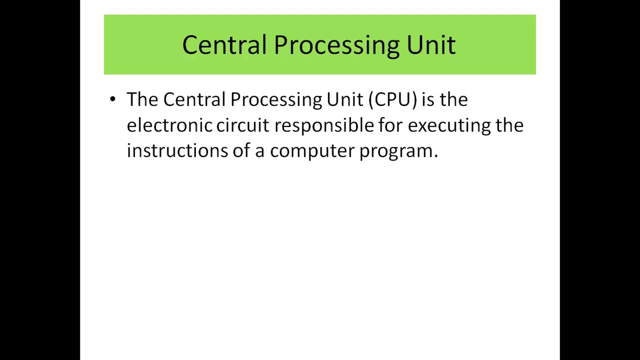 it has three main components, that is, alu, control unit and registers. so these are the units. that is cpu, which is further divided into two parts. alu and cu registers are there, buses, main memory and ru unit. let's start from cpu. so this is the full form of cpu. this is not complex cpu, so let's start with the Play button. now all SYK is staring into the Armory and usim remote functions. the usb drive partner. if you have B Natasha, central cmos is difficult toicking cpu or even근 capital c movies, life on the. 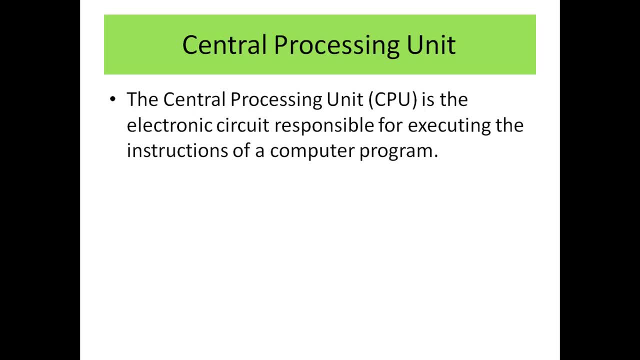 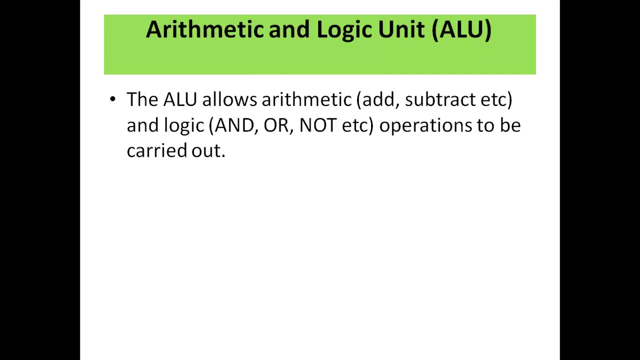 CPU, that is, central processing unit. it is the electronic circuit responsible for executing the instructions of a computer program. it is sometimes also referred to as the microprocessors or processors. also, the CPU contains the ALU, CU and variety of registers. so first of all, ALU. this is a main part of CPU. so the ALU allows us to perform various types of operations. 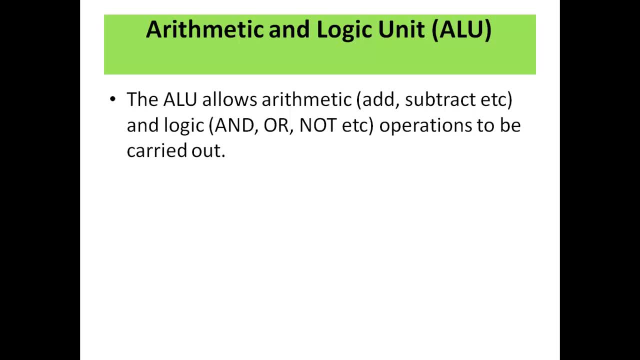 like automatic operations, logical operations and relational operations. we also have some electronic circuits in, available in ALU, like adders and subtractors, with the help of which we can perform addition and subtraction. we do have some division and and ending operations, also for logical operations- ending, oring or XOR or shift operations also. so all these 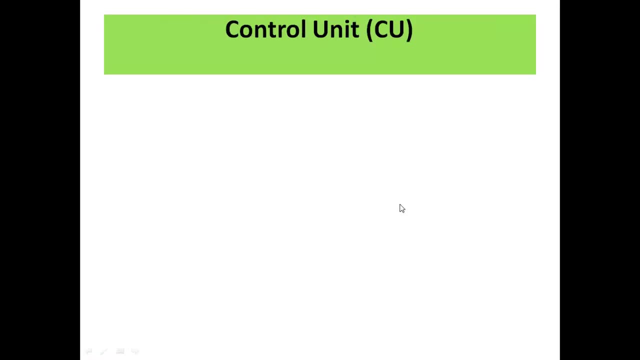 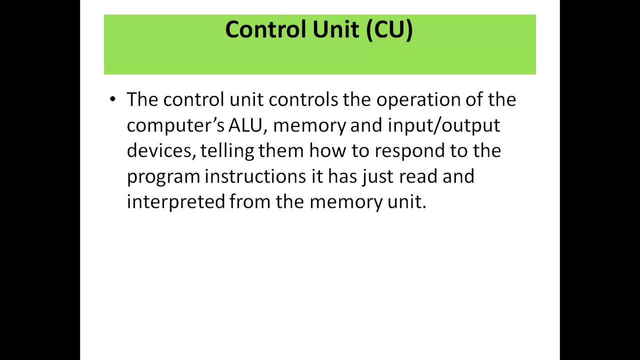 electronic circuits are available in ALU. another part of CPU is control unit. control unit controls the operation of the computers, ALU memory and IO devices telling them how to respond to the program instruction it has just read and interpreted from the memory unit it maintains. it maintains timing signals. 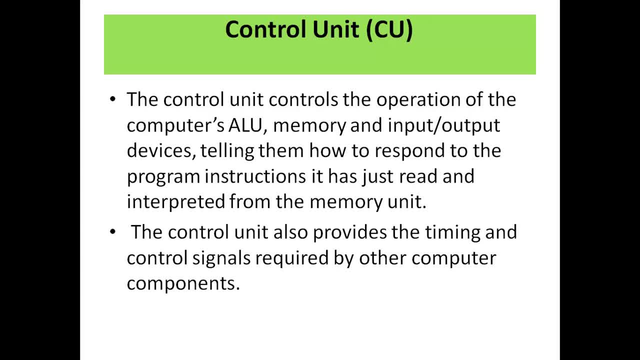 and control signals. also, timing signals will manage the timings. that is what type of instruction executes first and what instruction run next. let's say in our program we have 10 instructions, then what is instruction? what instruction has to execute first and what in the last? all these are basically managed by it. let's take the. 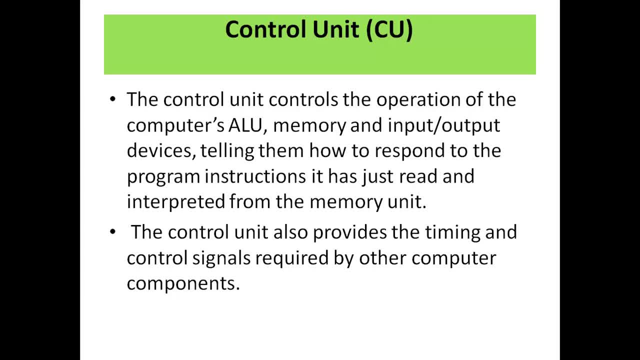 example of driving car. the instructions for driving the car is: first of all we have to press the clutch first, then we will have to change the gear, then give raise. we can. we can't change these type of sequence of instructions or steps. we can't change these sequences. so to keep track of this we need a dedicated 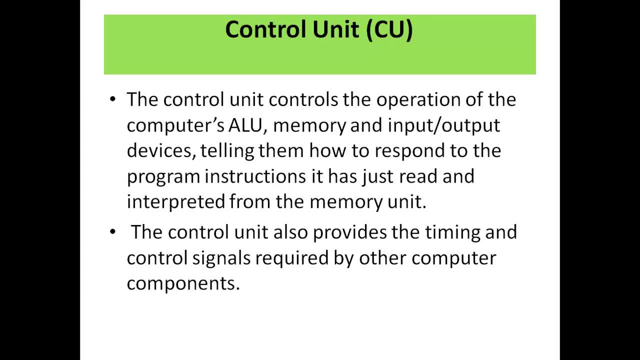 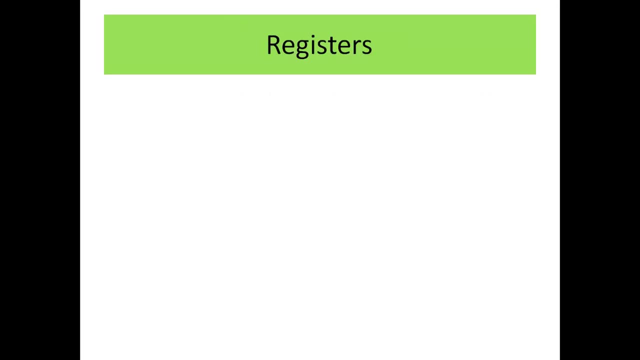 hardware and that hardware is and that hardware is control unit. so timing signals are basically used to generate timing and at every timing we have to perform one predefined action. next we will move towards the registers. you can see, registers are high-speed storage areas in the CPU. all data must be stored. 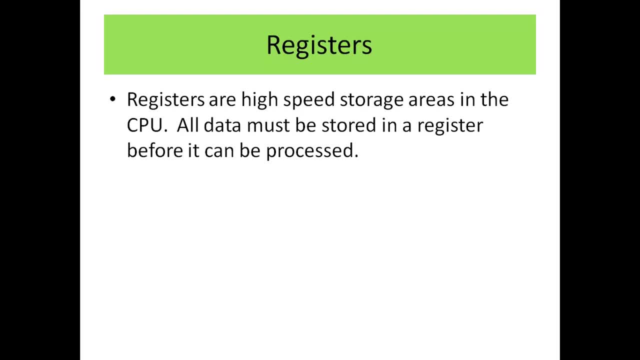 in a register before it can be processed. registers are the fastest available memory and contains the temporary data data and of very small size. it has of, let's say, 8 bit of size. the important point is that why we are using the register even when we have the main memory. so the answer is: speed means all. 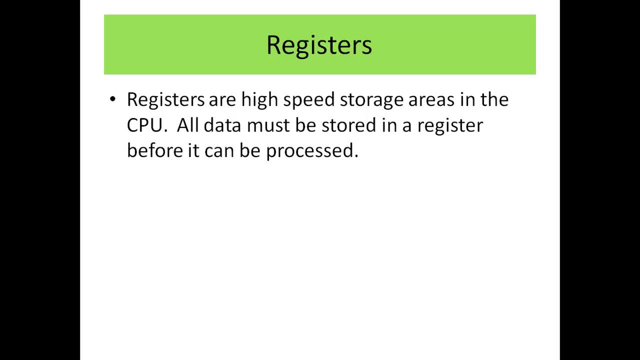 those operations which we have to do in order to use the register. we have to do, all those operations which we are performing, like a is equal to B plus C. all these data are available in main memory, but it has to perform in ALU and the speed of ALU is very fast and in comparison to the speed of ALU, the 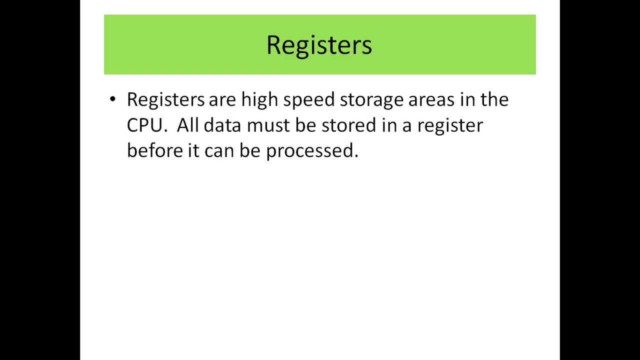 assessing speed of main memory is slow, so in the result of speed mismatch are there, then the burden of our load is on ALU. so here comes the role of registers. they keep in intermediate results and store some IO data temporarily. all the there are different types of registers are there, like ma register memory��. 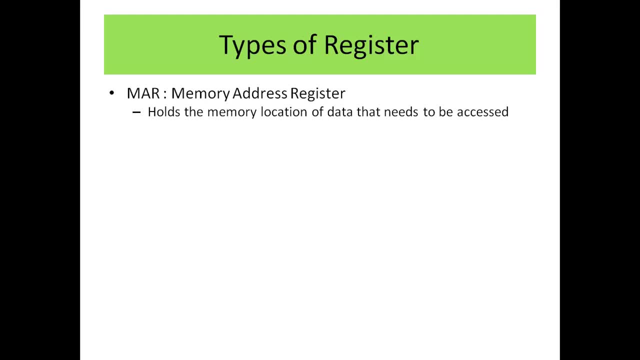 regulators: memory address registers. that holds the memory allocation of data that needs to be exist. next, MDR memory data registers are there that holds the data that is being transferred to or from main memory. next is accumulator, where intermediate automatic and logic results are stored can. these are some types of registers are. next one is program counter that. 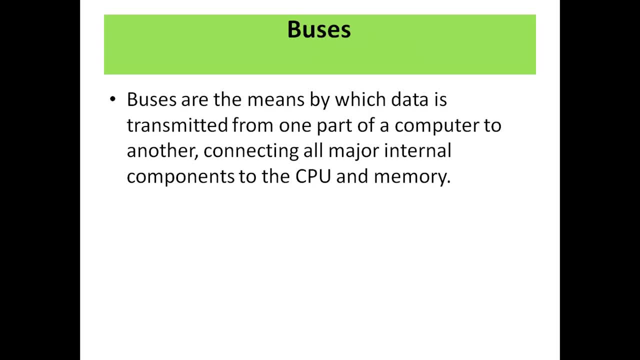 contains the address of the next instructions to be executed. next, the component is buses. it is very important component with the help of which we can transmit our information from one place to another, basically between CPU and main memory. these are some types of buses, that is, address bus which carries 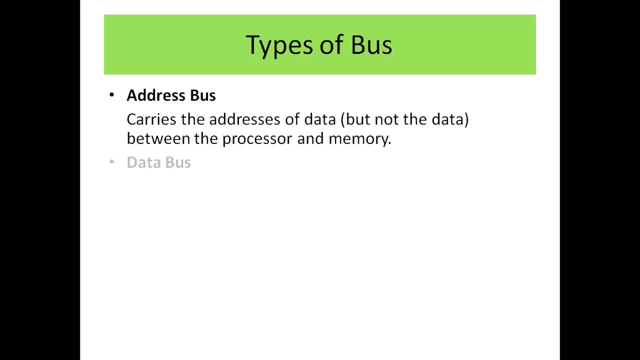 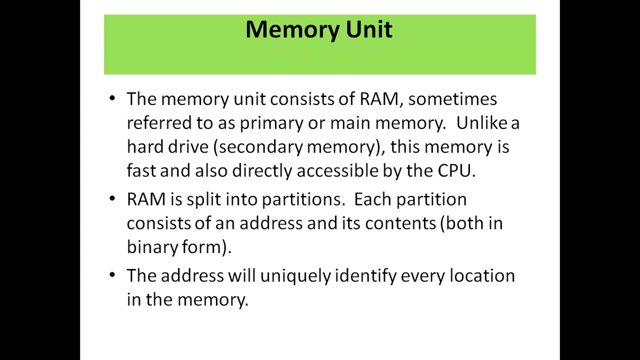 the addresses of data between the processor and memory. data bus that carries data between the processor, the memory unit and the input output devices. next, we use the control bus also that carries control signals, commands from the CPU, status signals from other devices, in order to control and coordinate all the activities within the computer. next unit is memory unit, the. 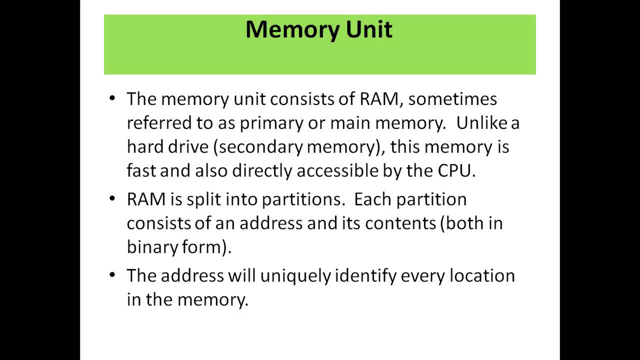 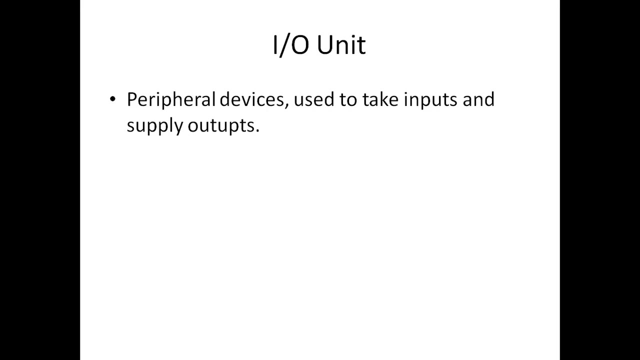 memory unit consists of RAM, sometimes referred to as primary or main memory. unlike hard drive, this memory is fast and also directly accessible by the CPU. RAM is split into partitions. each partition consists of an address and its contents. they, the address, will uniquely identify every location in the memory we do have. I would units also the. 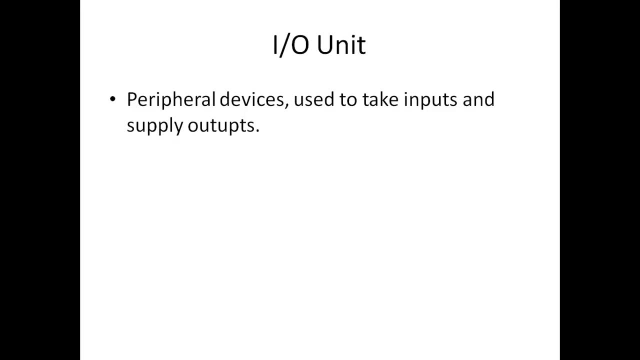 responsibility is to take inputs from from the outside world and supply outputs to the outside part. now we will moving towards the Harvard architecture, which is somewhat different from the Von Neumann architecture. the Harvard architecture has physically separated storage and signal paths for instructions and data. in the Harvard architecture, 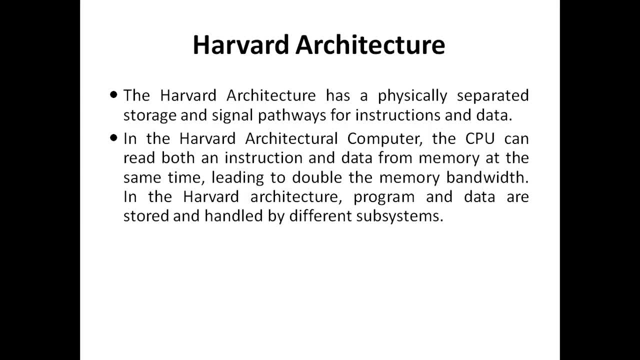 computer. the CPU can read both an instruction and data from memory at the same time, leading to double the memory bandwidth in the Harvard architecture program, and data are stored and handled by different subsystems. example includes microcontroller based computer system like single chip microcomputer and digital signal processors based. 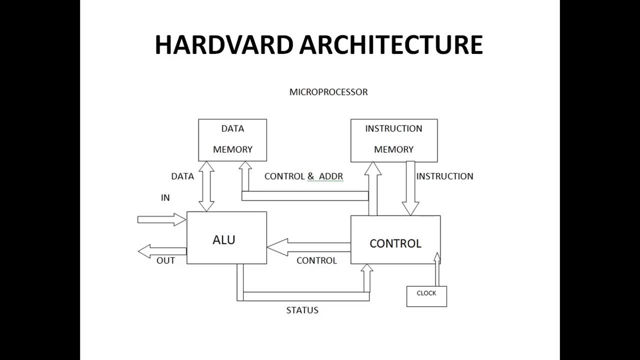 computer systems. this is the diagram of Harvard architecture, where we can see that memory is divided into two parts. these are means, these are the different memory locations, or we, we can say that we have created a different memory for containing data and different memory for instructions and all these instructions. 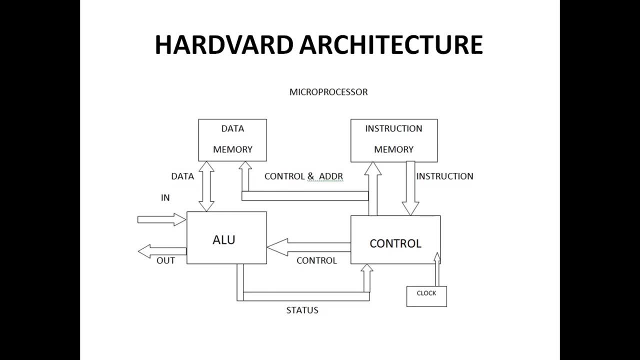 all these memories are controlled by the control unit, control unit and you can see that, you can see in the diagram that if we, if we need data, so data is connected to different buses and instruction is connected to the different buses means it can, it can, it can create a large speed in the Harvard architecture. a. 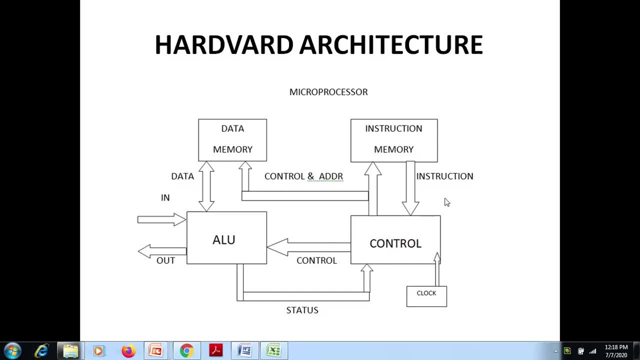 microcontroller with Harvard architecture can both read an instruction and perform a data memory access at the same time. even without a cache, a Harvard architecture microcontroller can those be faster for a given circuit. complexity because instruction fetches and data Access do not content for a single memory pathway. so we conclude.